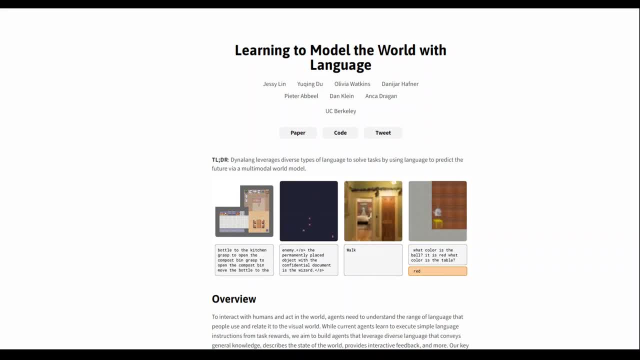 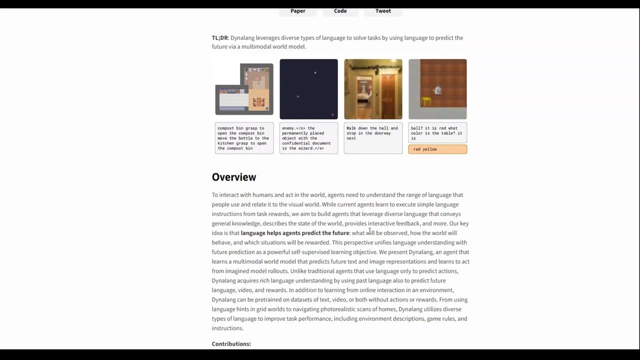 that the language is a tool that helps agent predict the future, and that is where this paper merges language comprehension with future prediction, serving as a great tool for self-supervised learning goal. In this paper they have introduced something called as Dynalag. this Dynalag is a sort of- uh, you can take it as an agent that learns, a multi-modal 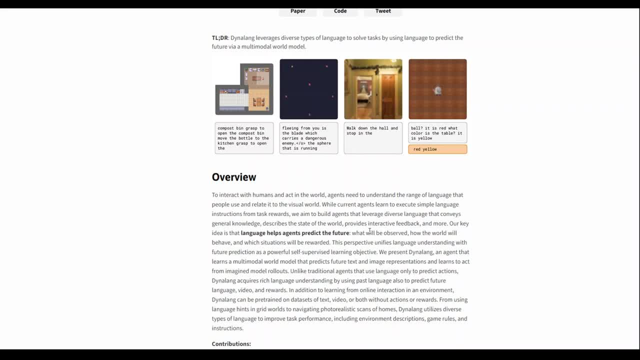 world model And it also predicts a future text. plus, it learns actions based on 功能. This paper question immersion zen, Flowardschool, the future Zoo, nida lag, is sort of you can take it as an agent that learns a multi-modal world model and it also predicts the future text. plus, it learns actions based on. In gdzieś ke therapy, hogy mộtrito te è Particularly a loong130 student. Lulectivond Dani Lu causa vos Mercing from future text. In this paper they have introduced something called as Dinah lag. This dinah lag is sort of you can take it as an agent that learns a multi-modal world model, and it also predicts a future text. plus, it learns actions based on. 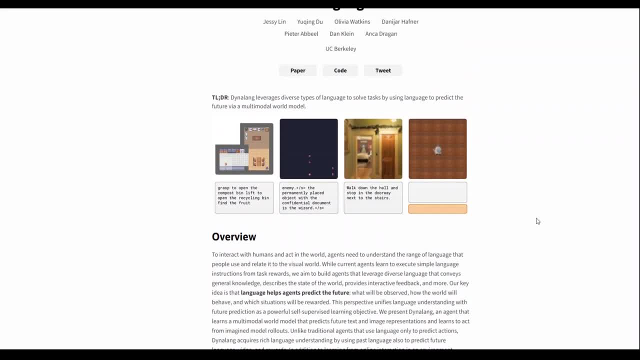 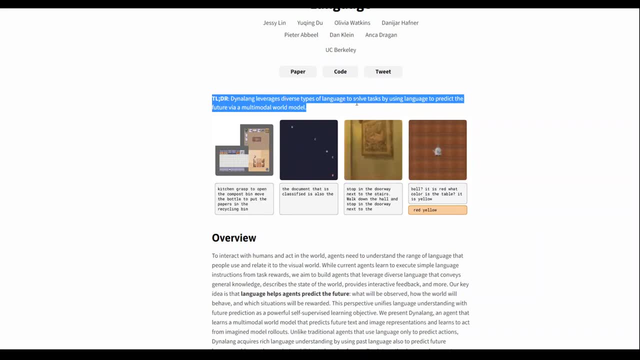 imagine, imagine, model rollouts. now this: they have this tldr here which you can read through that dynalang leverages diverse types of language to solve tasks by using language to predict the future. um, now, another thing is that: what exactly separates out this dynalang? 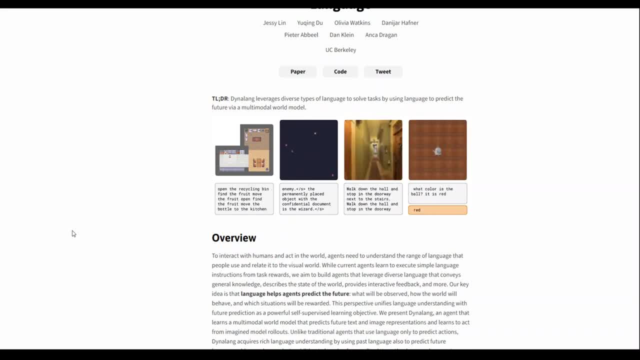 from others. there are other agents too, but what dynalang does is it uses past language to forecast future language, video and rewards. it can also be pre-trained on video, text or both, even without actions on the board, which is a great thing. there could be a lot of use cases for this. 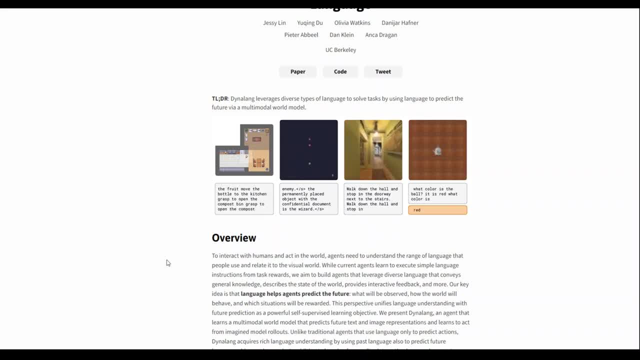 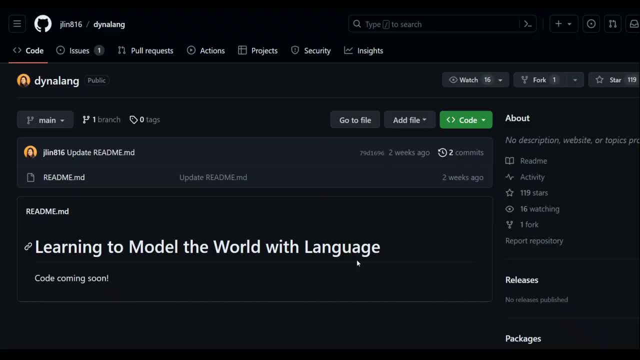 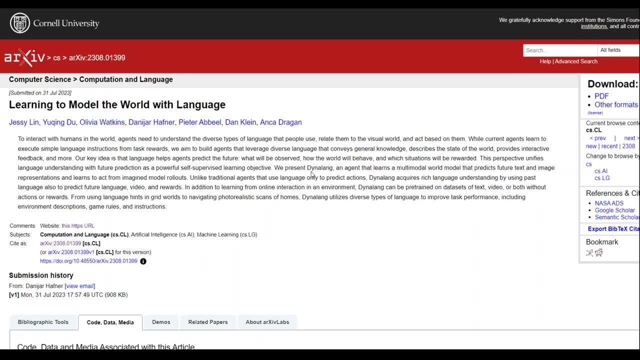 video description so that you can keep an eye on it. they also have this paper in here on it. they also have this paper in here on it. they also have this paper in here on um on um on um. on the connor university's website. where on the connor university's website? where.